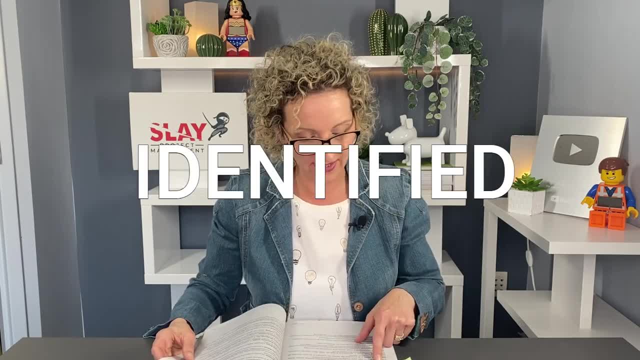 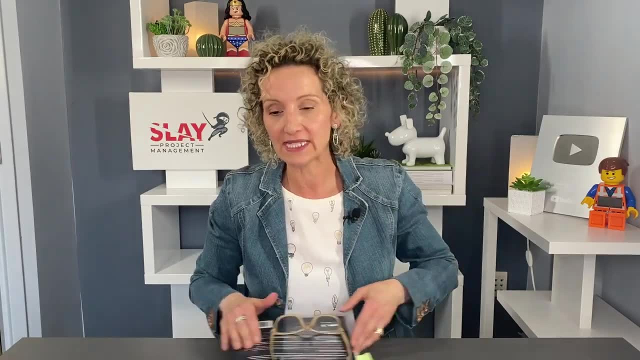 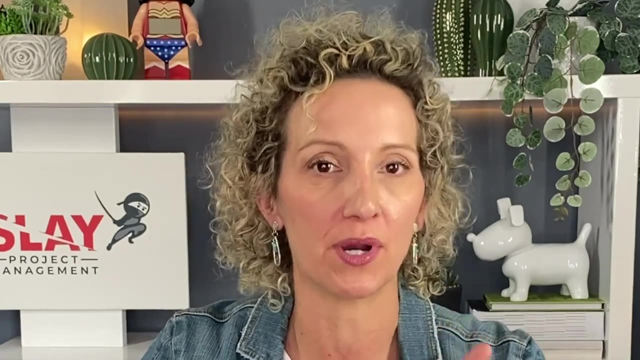 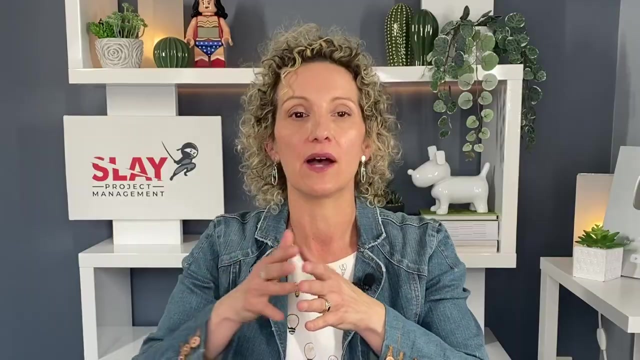 or baselines associated with the project are identified, documented, approved or rejected. Okay, so what does this mean? It means that anything that you change to your approved baseline project plan ought to go through some sort of change control management. Now, things to look for and how I kind of really just make it really easy, is 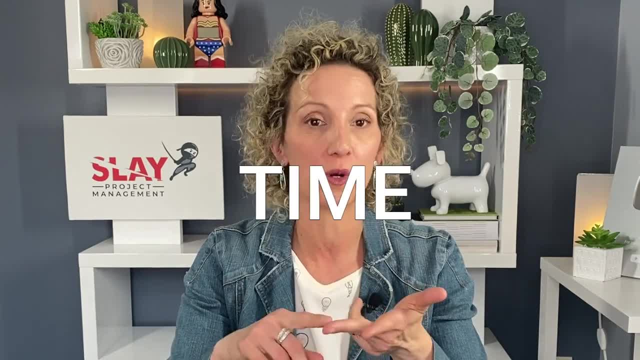 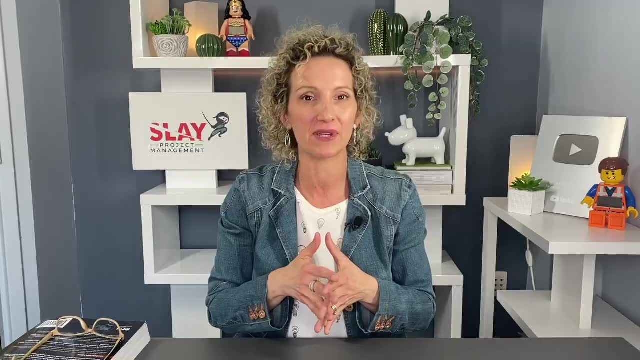 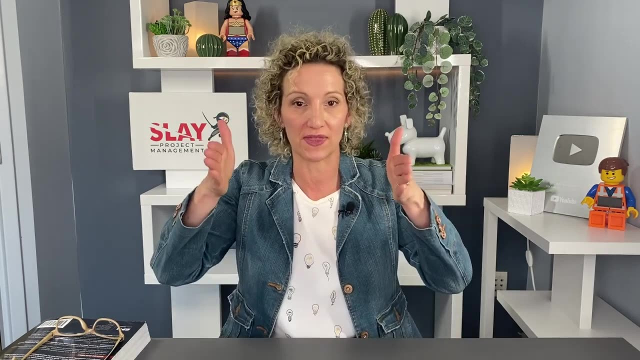 anytime I'm looking to change scope, time or budget, that is going to impact and be a shift from a normal parameter because again you can have shifts inside your timeline that you don't have to go through change control because you're just shifting within the set. 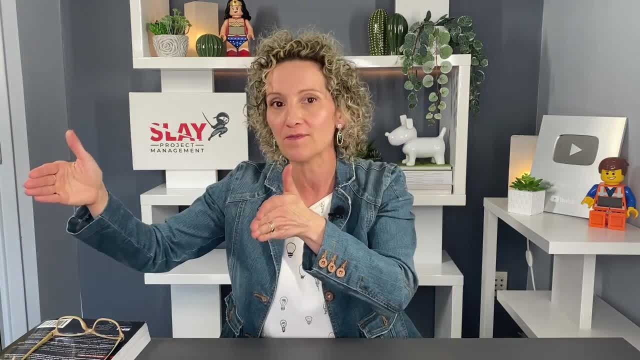 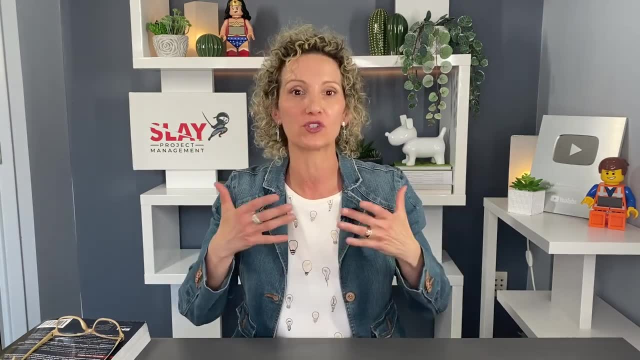 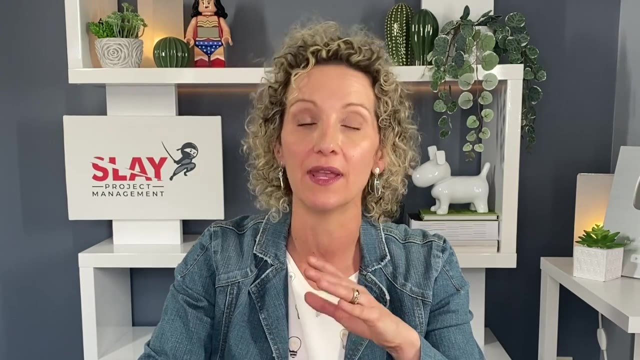 time. So if you're now moving that parameter or for a budget, you have an amount and you now need to ask for more or for the scope you want to add more to it. guess what? You need change control. It is so easy for someone to say to you: hey, can. 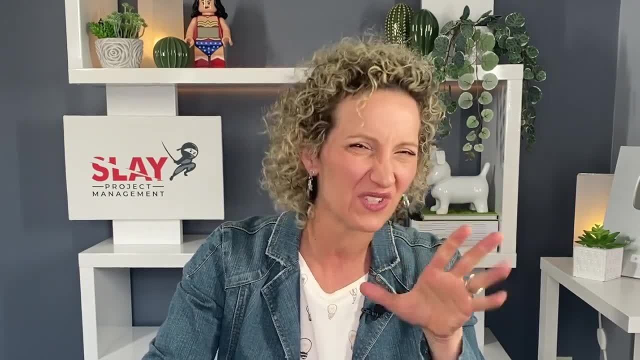 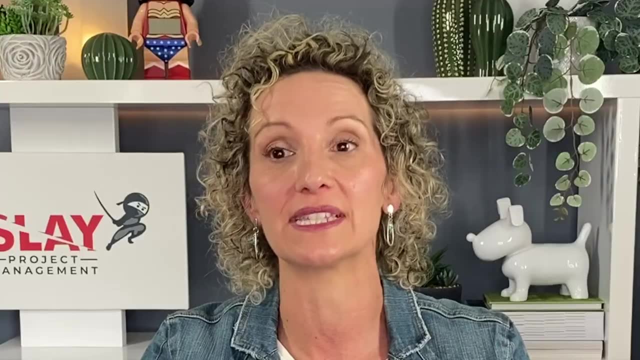 you just add that to this, please. It's gonna be really simple, extremely easy. but what they don't realize is that simple request can actually lead to an increase in timeline, pushing out your go-live date, actually having more impact to your deliverable. 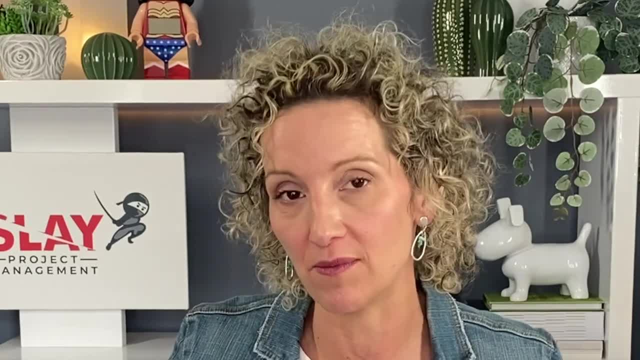 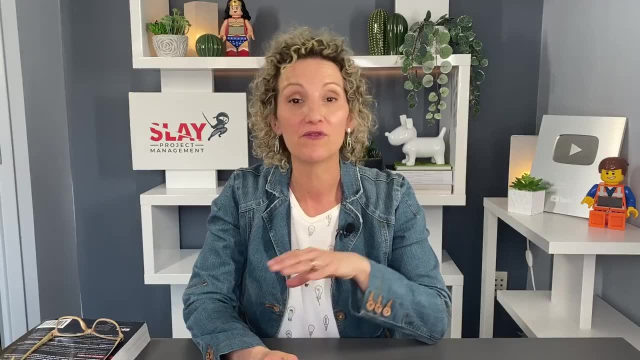 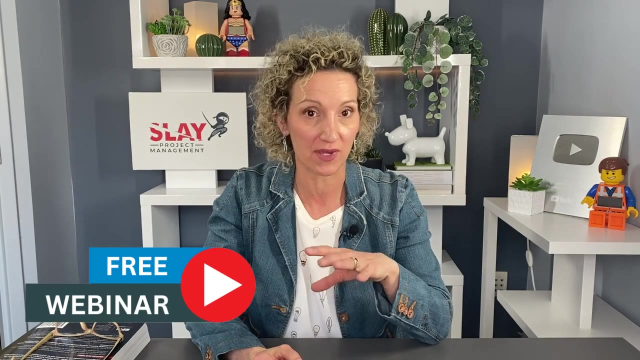 maybe costing more money, and where are you gonna get that budget from? So project change control is super, super important. Before we move on to talk in more depth about change control, I have a free webinar on the five fundamentals of project management that I highly recommend you check out. and guess what? 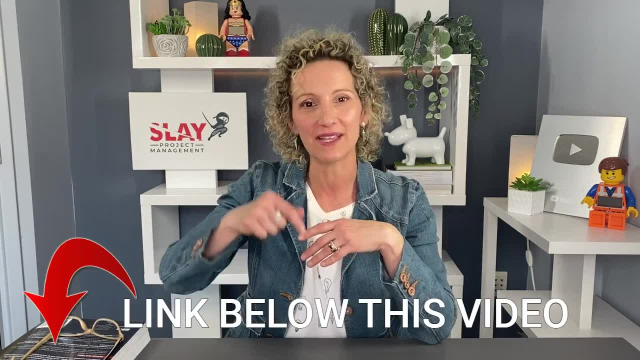 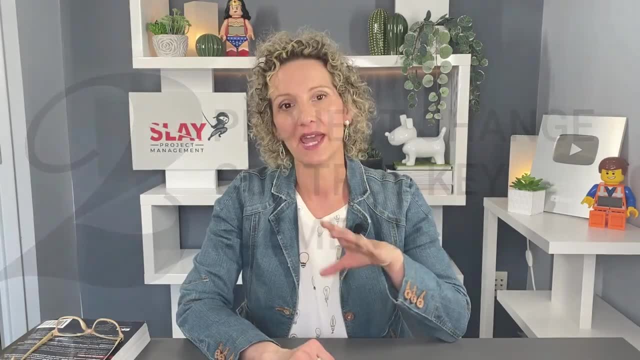 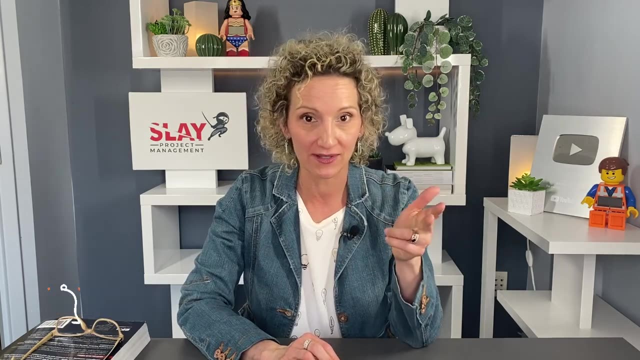 It's free and it's a webinar and you can get it from the link below this video, So definitely go check it out. Project change control: key elements. Now there are four distinct key elements when it comes to project change control and ensuring that your scope, time and budget stay on track and that you're analyzing. 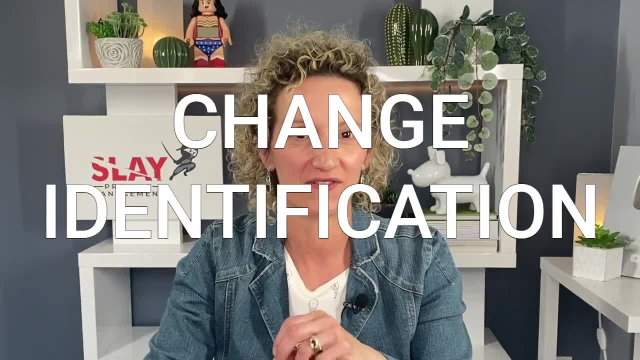 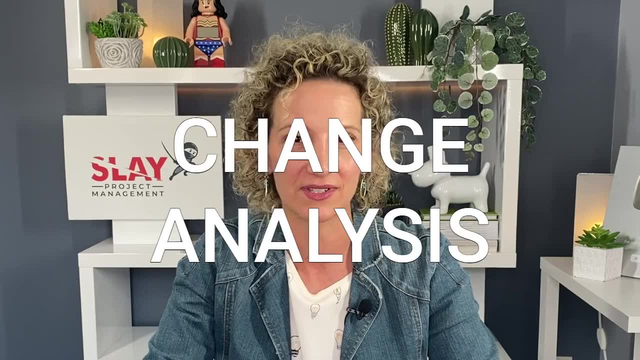 it properly. So the first one is change identification. You want to have an understanding and identify what exactly is the change that is being asked Change analysis. Once you understand that, you're going to be able to do a lot of things. You're going to understand what's being identified and what's being. 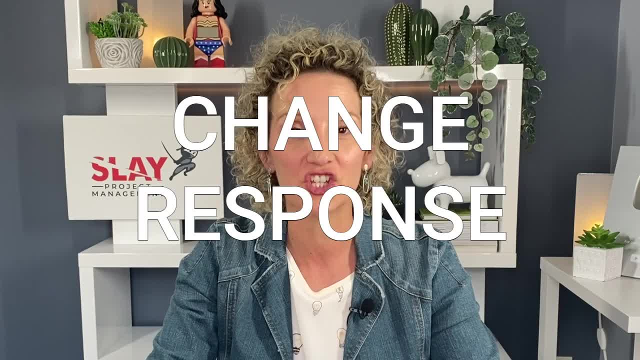 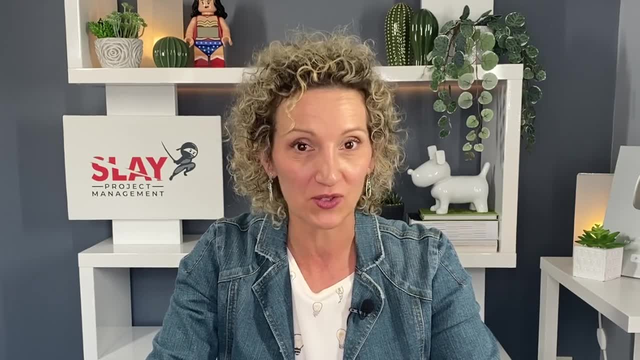 asked of you. You now just have to analyze it to understand the impact Change response. Once you've done the analysis and understand if you're going to take it on or not, you now have to respond to it. Are you accepting it? Are? 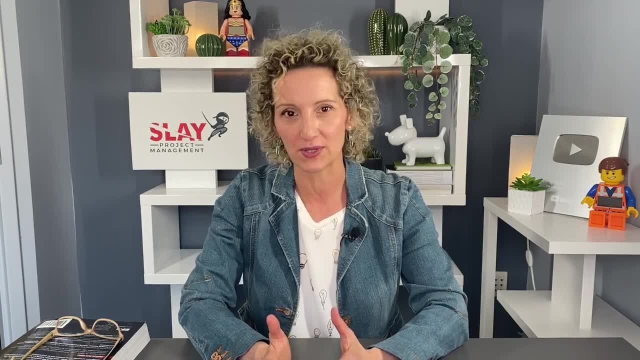 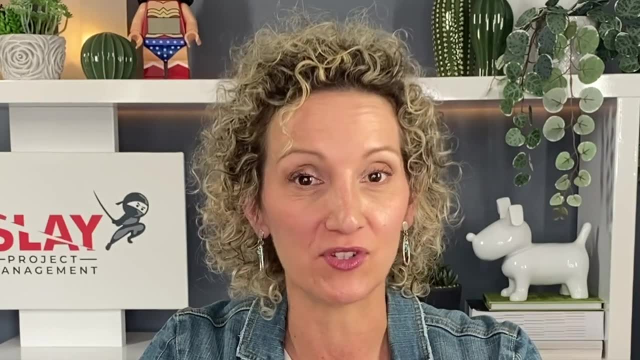 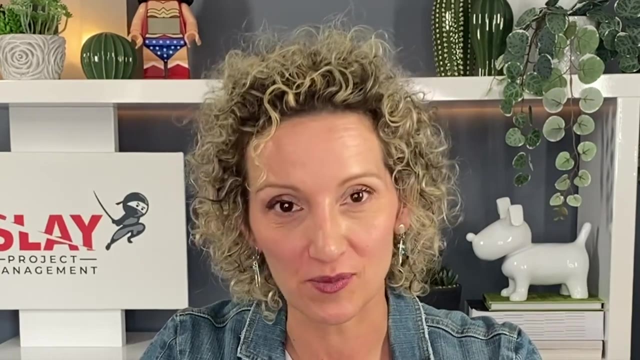 you rejecting it? Are you still going to be thinking about it? That becomes really important too. And the last is change communication. You need to now communicate. what exactly have you decided to do? Are you accepting it? What's happening? Who's impacted? Do you have to do another rendition of your project? 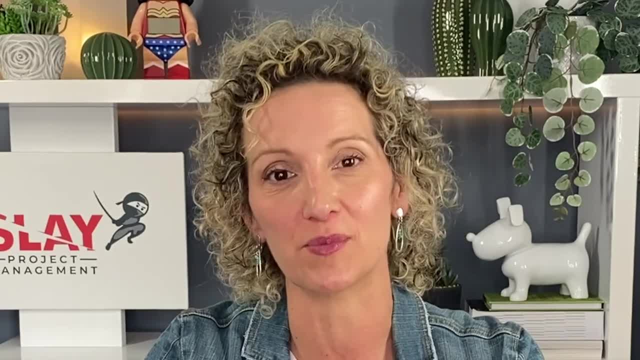 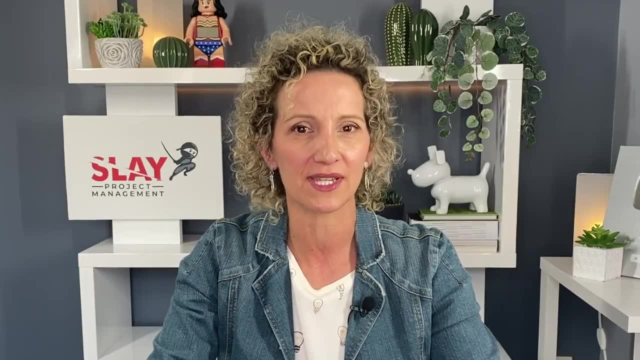 plan. If it's being declined, why is it being declined? Allowing for the person who initiated that request to let them know that it's been declined Again. those are the four key elements when it comes to change control that you need to. 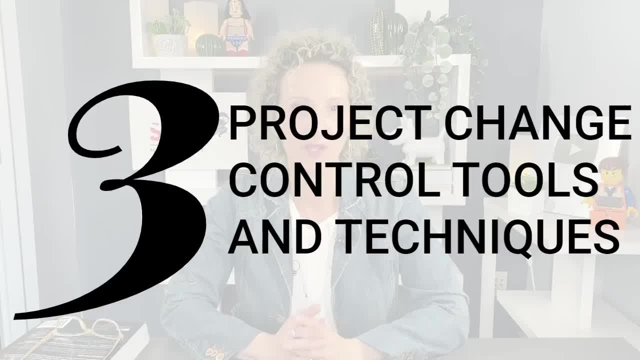 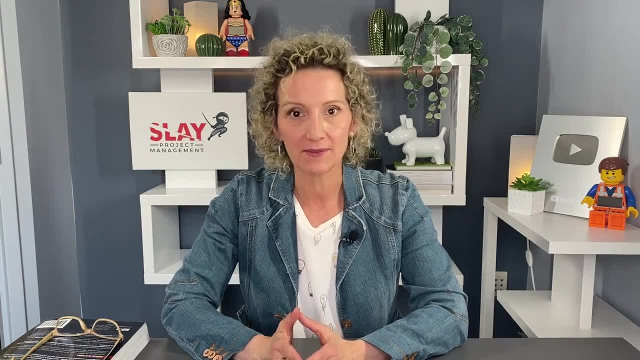 ensure that you go through, from a process perspective, Project change control tools and techniques. Now, I like to keep this simple, because sometimes when we think of change control, it feels extremely ominous and it's like, oh my goodness, this is going to be. 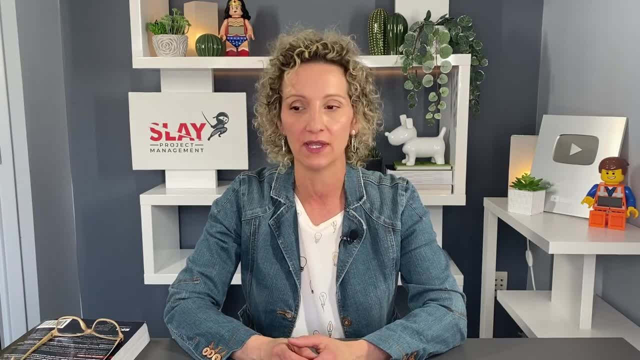 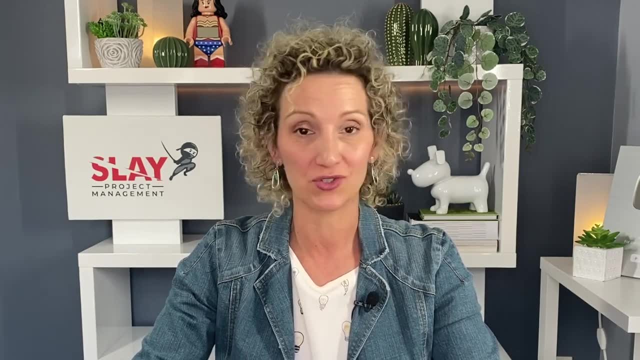 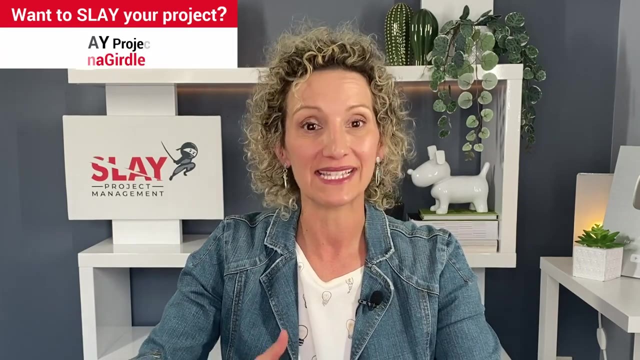 extremely paper-heavy and a lot of work, And it doesn't have to be, If you understand tools and techniques and you make it very simple. and guess what? I streamlined it for you too, because I believe in that in my online project management course, Slay Project Management. Basically, it's about using it. 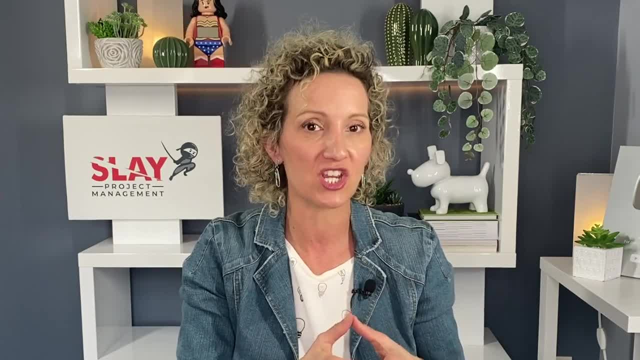 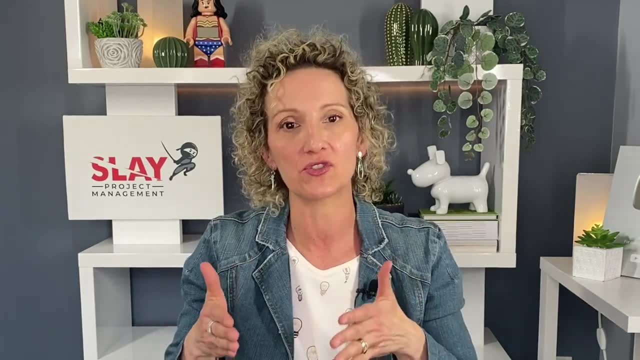 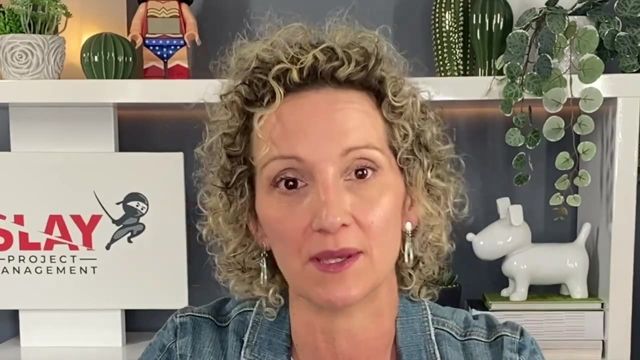 as a technique to make sure that people who are wanting the change truly want it for the sake of saying it and asking you for it And that, if the change goes through, you capture all your information. Remember, there's those four aspects you have to look at from a change perspective that I mentioned in the tip. 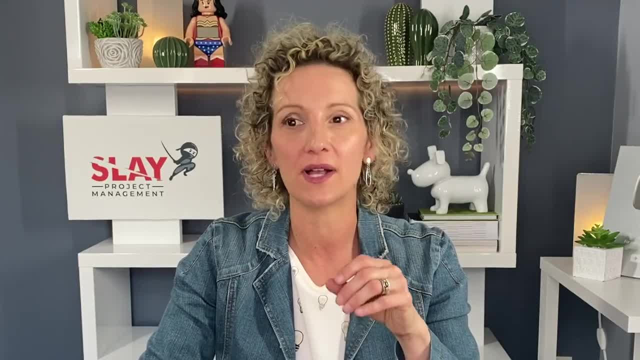 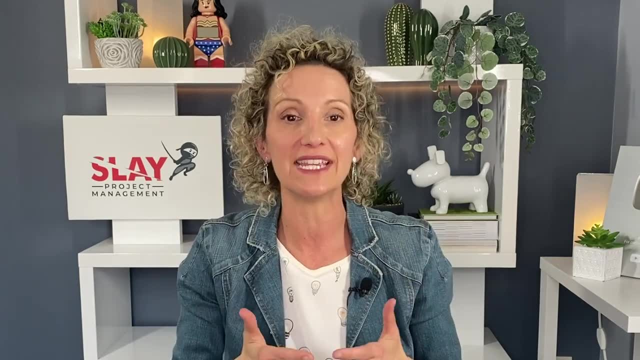 before. So what are some of the tools? Well, the tool is simply a- I call it a one pager. It's a sheet that has very specific questions that you need to ask the person who is requesting the change. What is your requesting? Why are you? 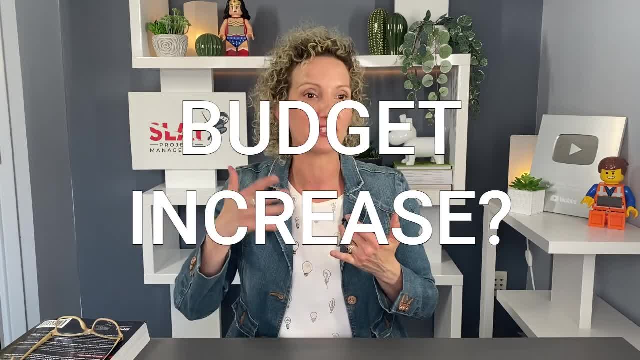 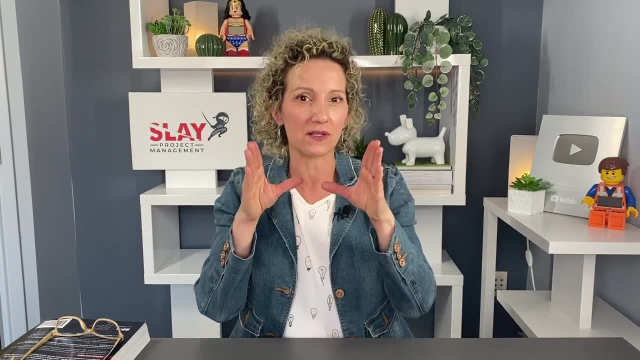 requesting it? What are the pros and controls? What are your feedbacks, What are your of that request? What is the budget increase potentially if this request goes through? Are there additional resources? These kind of key, fundamental things that you need to ask to ensure. 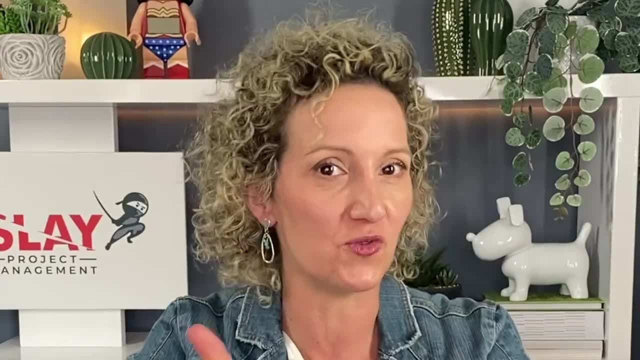 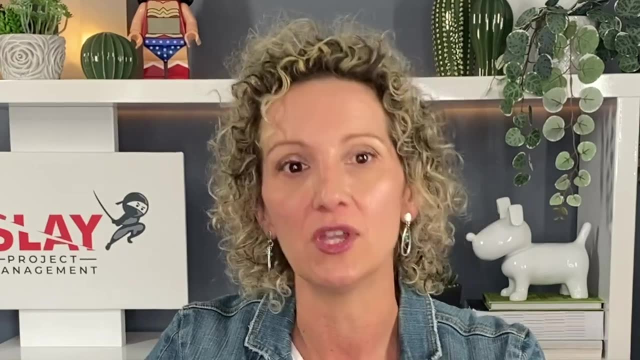 that you're really thinking it through, because if the change goes through, you need that information to make changes and update your project plan. But if the change doesn't go through, there's good reason why: because you have this information to really make good, solid decisions and pass that. 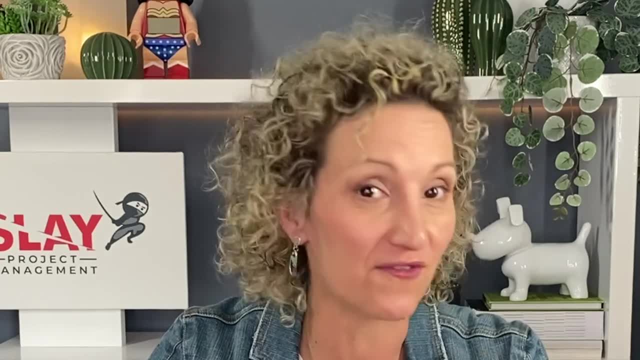 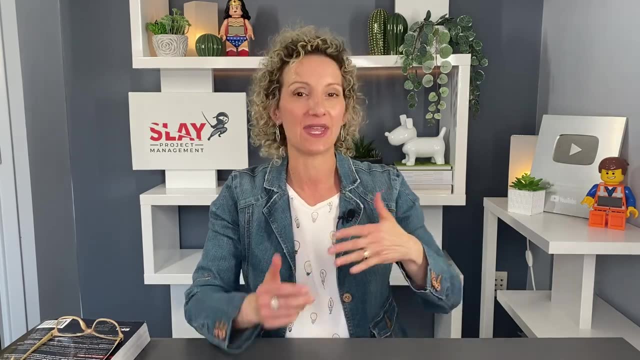 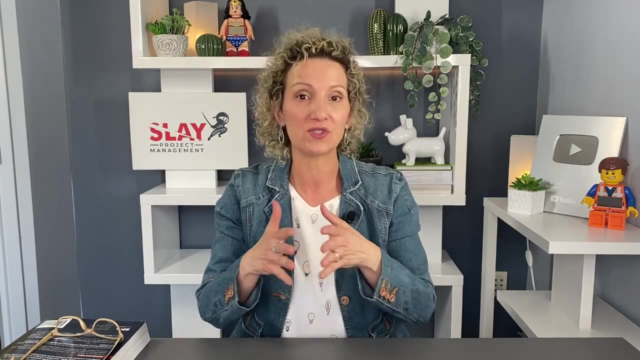 information along to your steering committee, who can give the final yay or nay. Now, when it comes to techniques, it's a process. So, yes, we have to identify it, analyze it, communicate on it, make decisions on it, but it's important that you also teach everybody what that process is. So I always 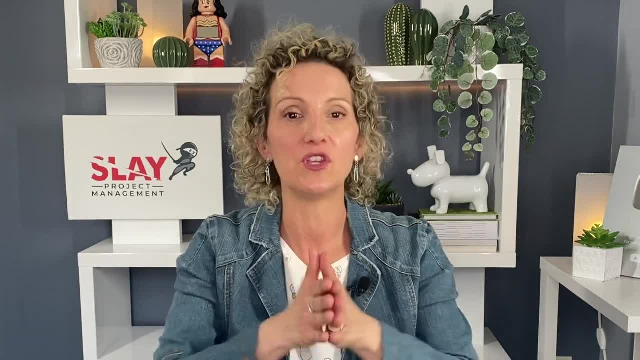 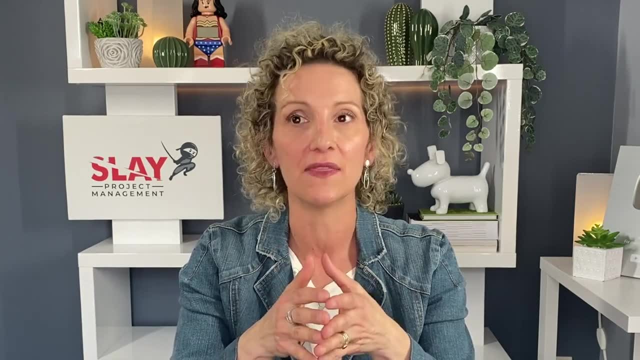 say to my team members and those and stakeholders involved: if you have a change and that change is within the current parameters that we have within the current parameters that we have within the current parameters that we have within this project, then we probably don't need a change control. but we still have to talk about. 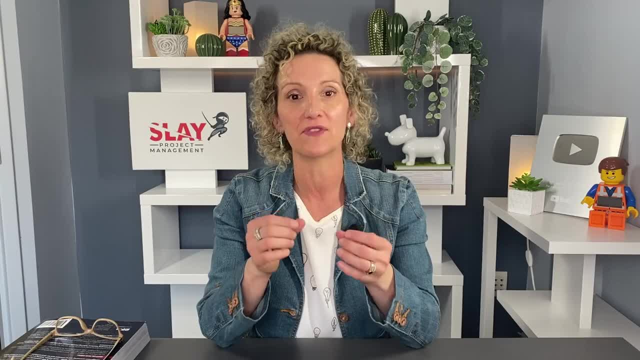 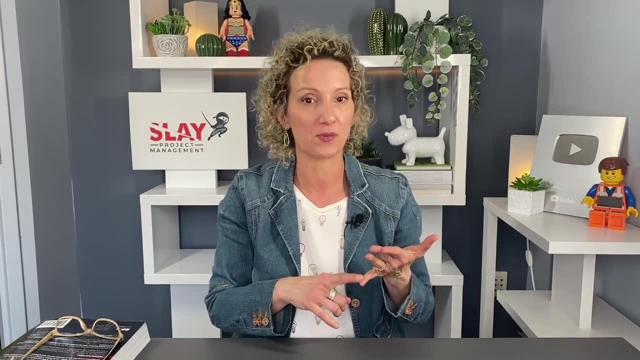 it as a team to understand what the impact is. But if there is a change that's going to shift scope, time or budget, then we have the process to follow. You have to identify it with the project team, bring it up at a meeting. You have to fill out the change control form that we talk about. 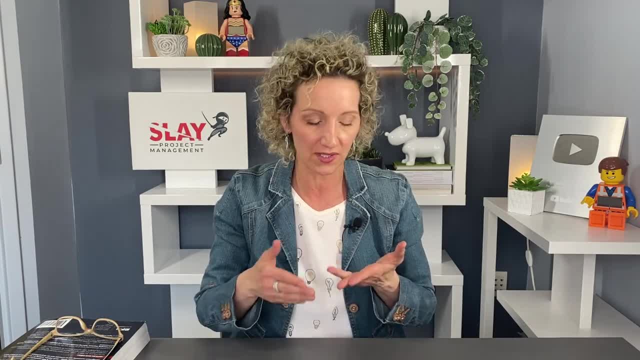 as a team, to make a decision collectively. is it really going to work? We then, if we decide that the something has to be escalated, we bring it up to the steering committee because, again, they're going to do all our work. they're going to do all our work. they're going to do all our work. 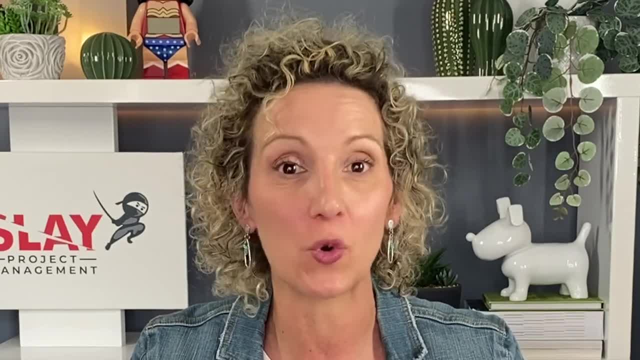 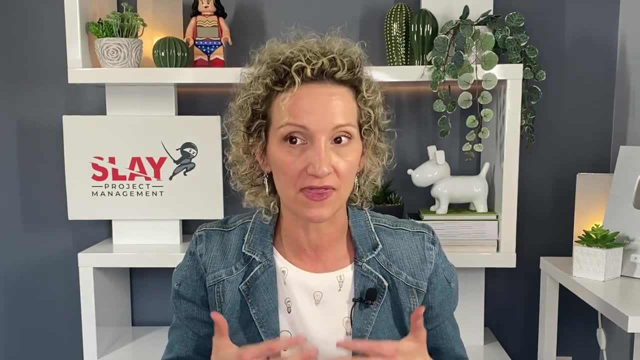 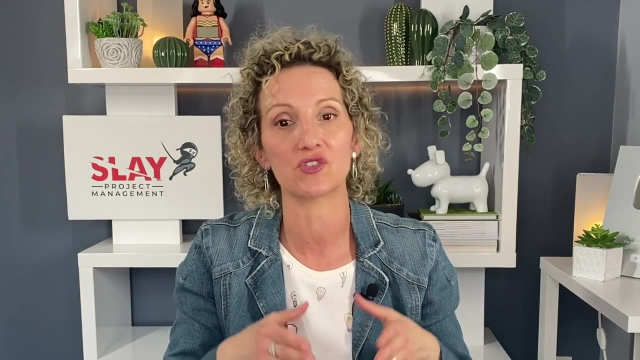 final approvals, particularly for something that may need more budget or may need an increase in time, But we as a team decided that it really was worthwhile and we should consider this particular change And then afterwards, you have to then implement it into your project plan and ensure. 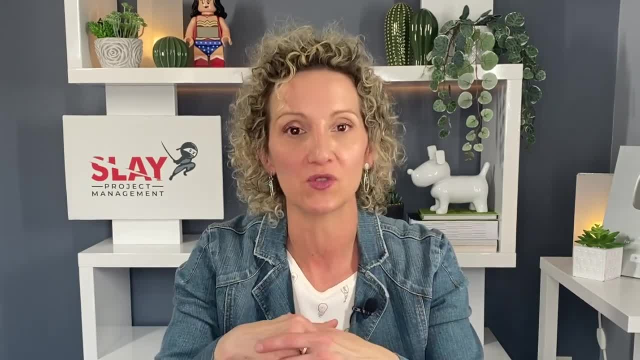 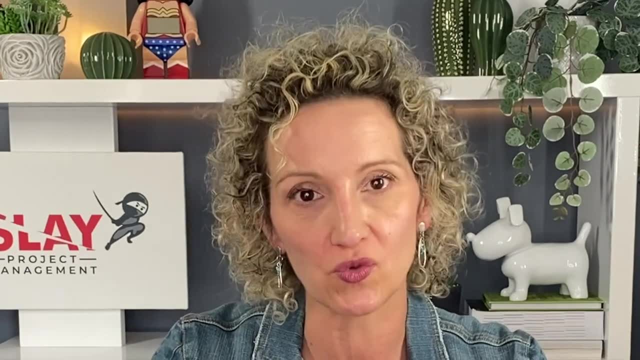 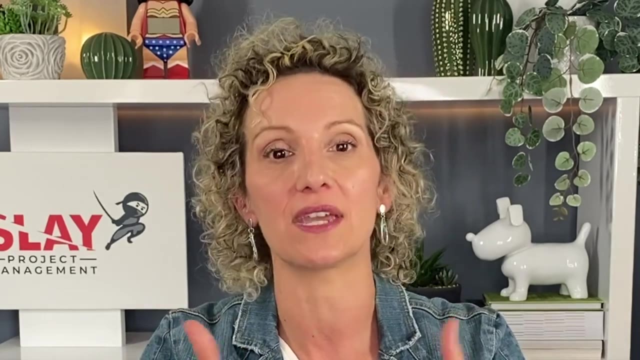 that those new tasks are distributed accordingly so you can start executing on it. So that's the process, the technique of implementing your change control, And the tool really is a simple one pager sheet document template that allows you to get all the information that you need. 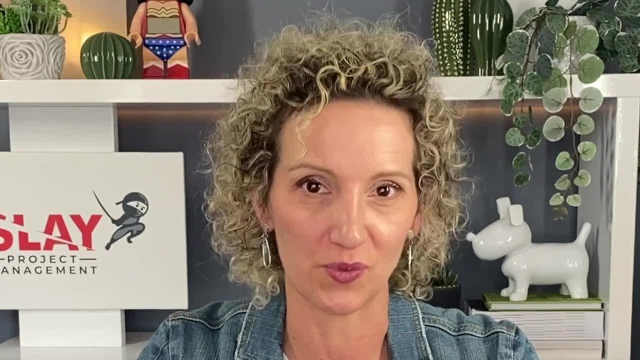 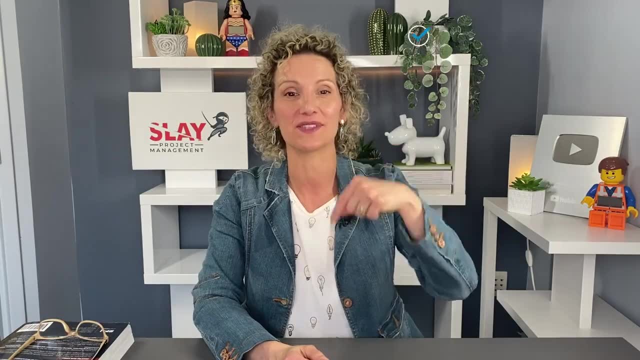 to successfully execute on change control in your project. Now don't forget to save your seat for that free webinar that I have for you. The link is below this video. Now, make sure you watch this next video, because you need to understand risk, because you're definitely going to have to look at.